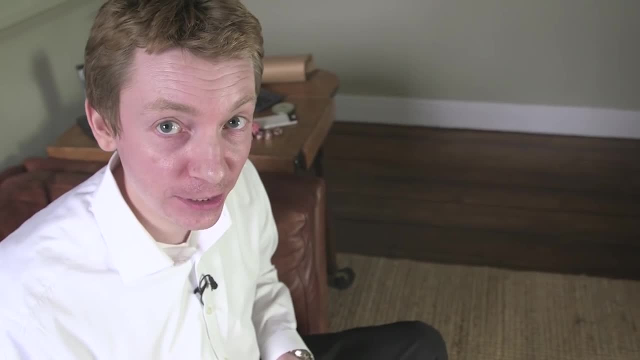 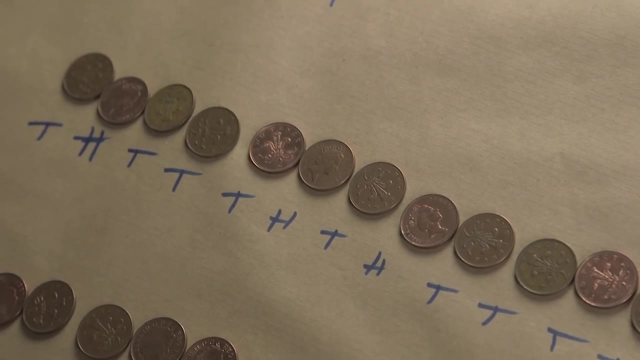 All right, we're going to look at this sequence and we're going to play the game where we're tossing a sequence of coins and we're waiting to see how long we have to wait for a head tail. If I start here, I'm looking for a head tail. oh, there, it is right. 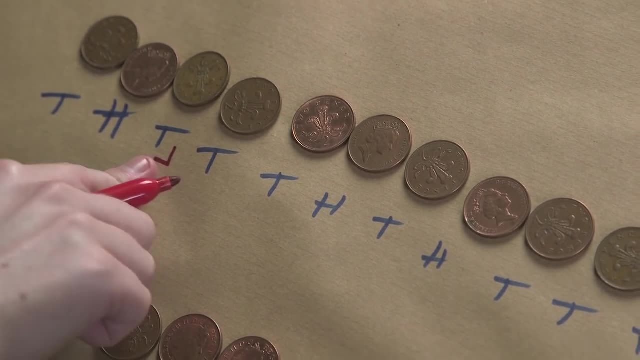 All right, that's my first head tail there. That was a waiting time of three And then I got head tail And then I start again. Okay, I do a new game. I'm going to look for head tail. 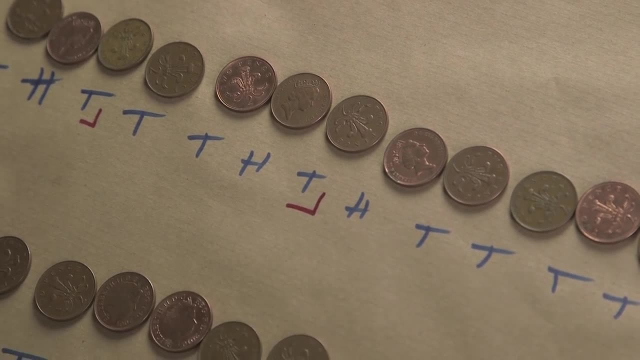 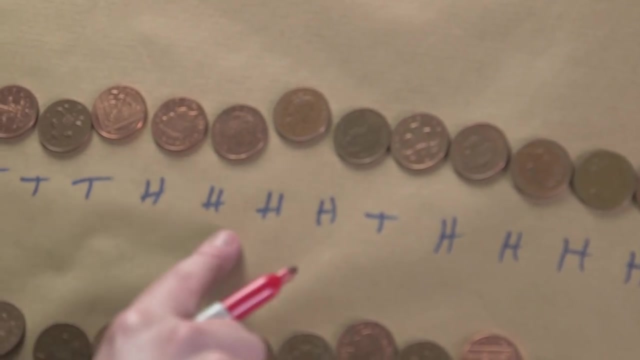 And I had to wait. one, two, three, Four. there it is. Now I'm going to do it again. Oh look, this one is straight away. Look, head tail. Now I'm going to start again. I'm looking for head tail. Oh, this is a long wait here. 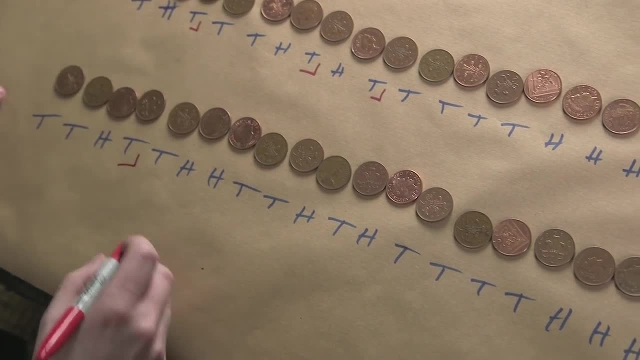 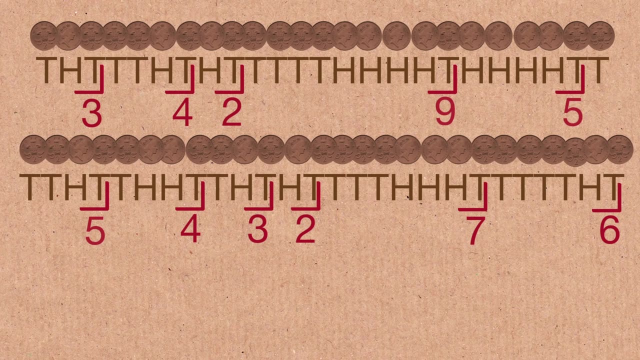 And then there it is, head tail, And oh, head tail there, There, there it is. Oh, there's one right at the end as well, Right? so what was the average waiting time? Let's have a look at the waiting time. 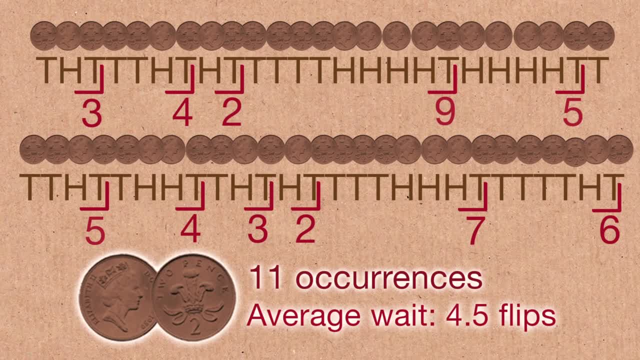 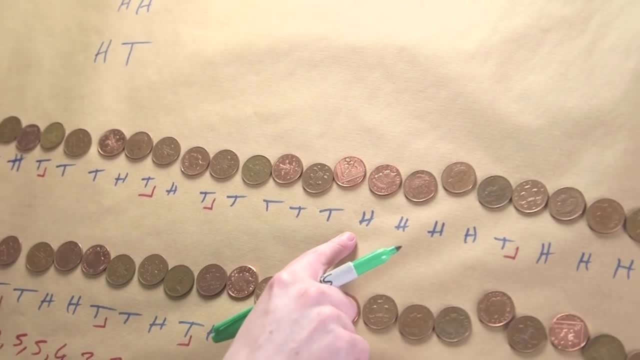 So that's about an average wait of 4.5.. Let's look at the heads. heads, though. You would have to wait. Oh how long. Oh, this is a long waiting time here. It happens all the way over here. 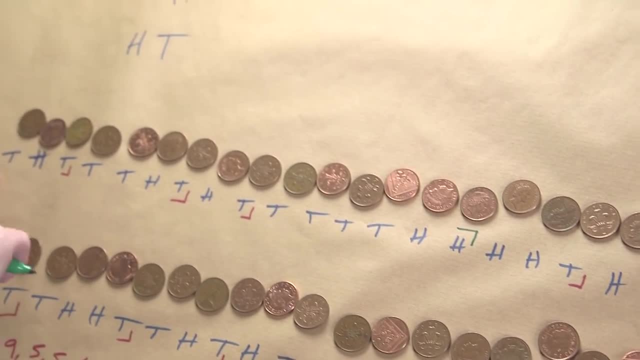 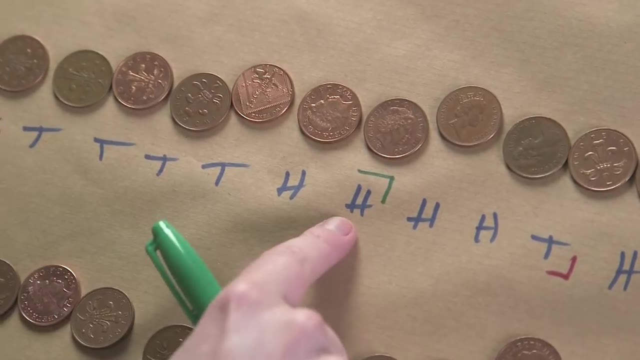 There Heads heads, which was a long wait. One, two, three, four, five, six, seven, eight, nine, ten, eleven, twelve, thirteen, fourteen, fifteen. So you've played a game and it ends when you get heads heads. 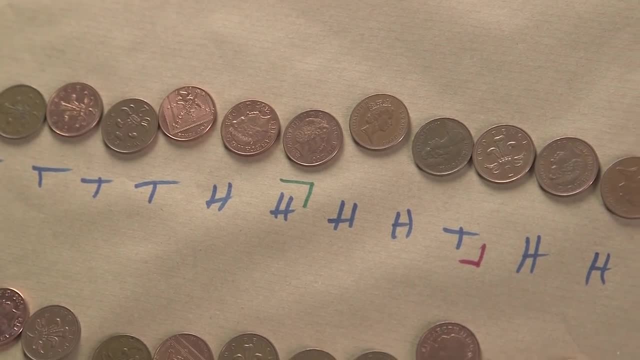 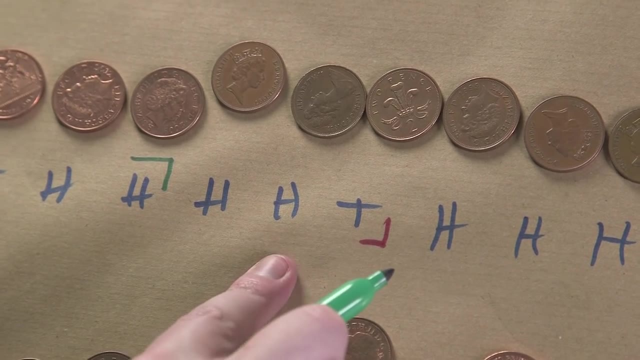 Great, done So. now we start a new game, a completely different game from this point on. So we'll just start again. Oh, but this time, notice the heads. heads comes up really quickly. Look at that, It's just straight away. look two. 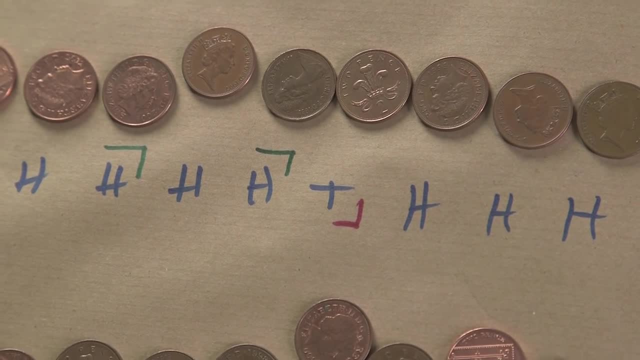 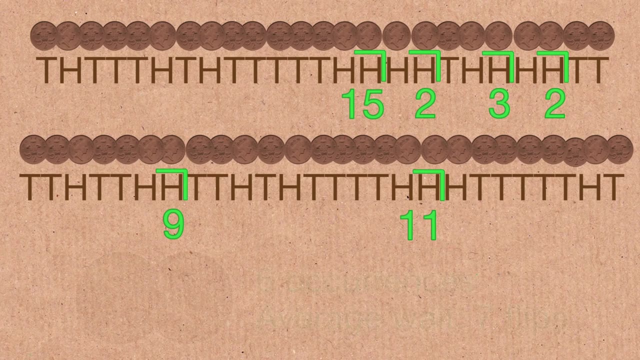 And now we start a new game. Okay, so we had a success. We'll start a new game and we have to wait One, two, three. Let's look for our average waiting time for heads, heads, Okay, which is seven, right. 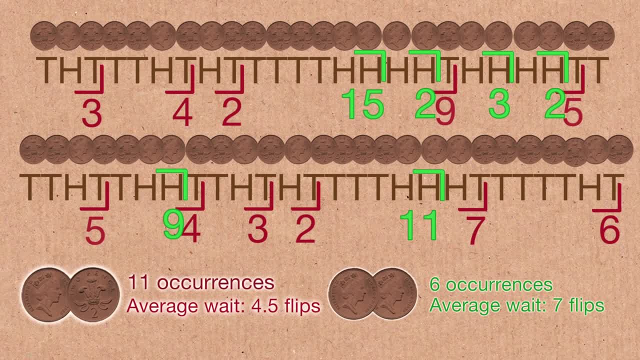 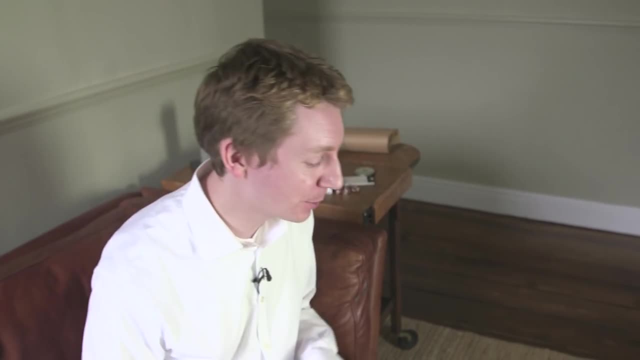 And yes, oh look, yes, You have a longer average waiting time for heads heads than you do for heads tails, even though they have an equal probability. They're both one quarter. Why is this? Because, if you noticed when we were doing it, 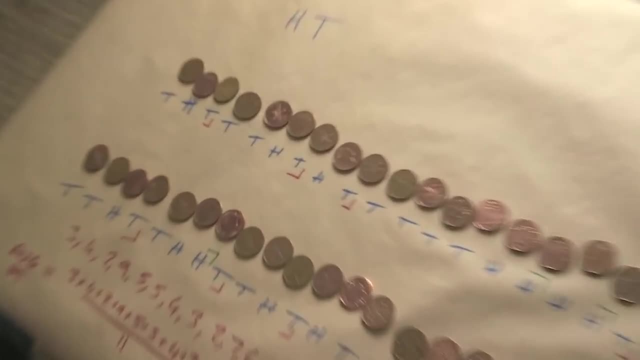 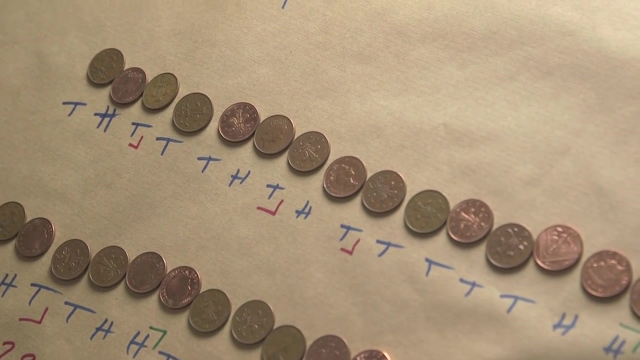 when you play heads tails, you get heads tails, then you start a new game and you wait for heads tails and you start a new game. heads heads was slightly different when we did it with heads heads. Look what happened here. 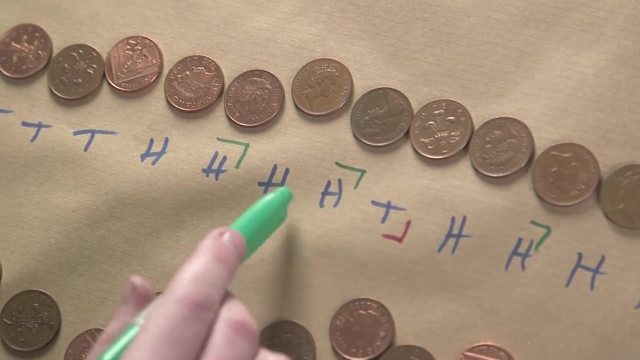 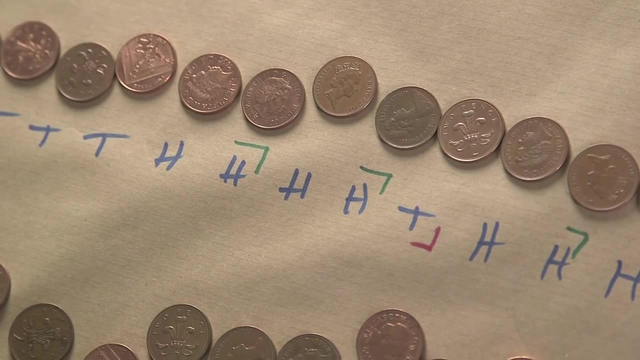 When you have something like this: heads heads, heads, heads, we have this overlap and this overlap isn't counted. We were playing it until we got heads heads and then the game stopped. We had to play a new game from that point. 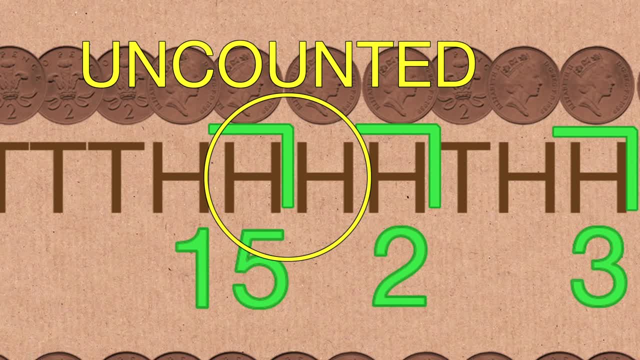 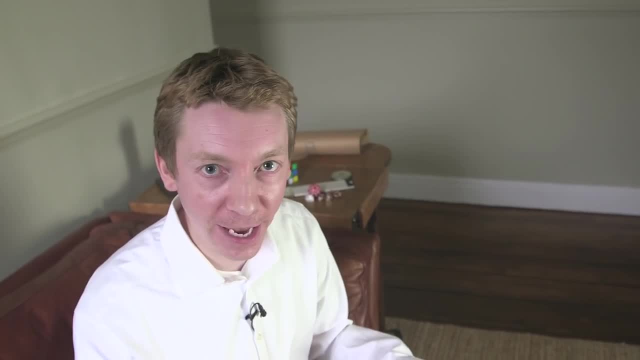 So here we've got a heads heads that didn't get counted as a heads heads. So if you look at how many heads heads we've got, it should be about an equal number to heads tails, but the overlaps don't get counted. 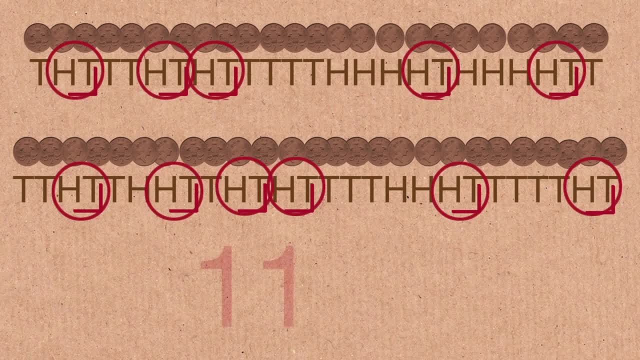 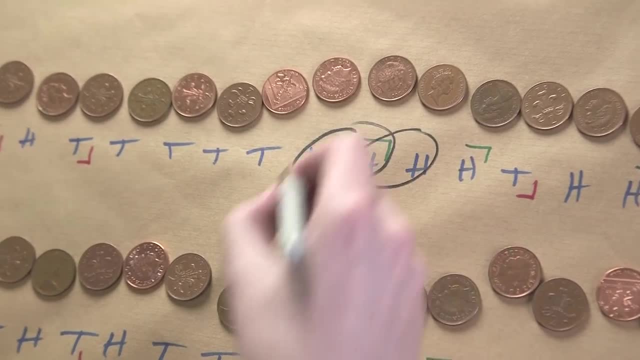 I mean, let's just check. So how many heads tails did we have? Well, actually, no, we got 11.. I know for a fact, we got 11.. How many heads heads did we have, including the overlaps? 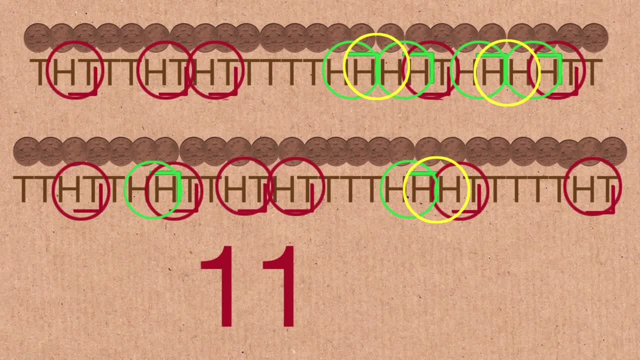 One here, we have two, we have three. So if you actually count up the heads, heads and tails, you can see that we've got 11 of them, but only six were included in our waiting time average, So this sequence- 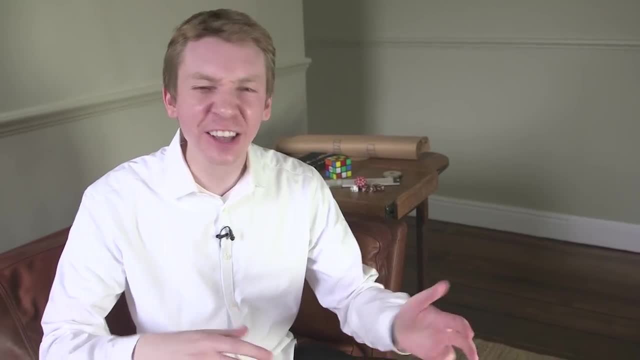 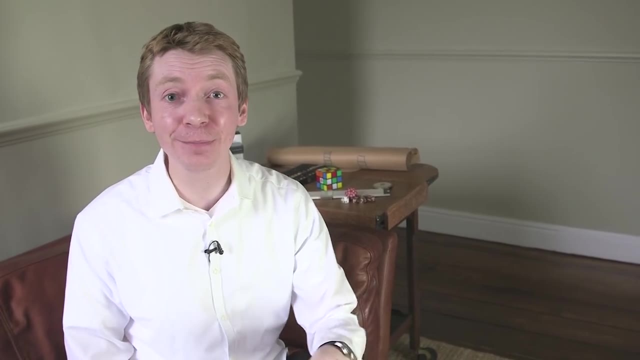 we were looking at what would happen for consecutive values. So you know, heads, heads, heads tails. The same sort of thing would happen with tails heads and tails tails. We're looking at consecutive values. In fact, the reason I mentioned this- 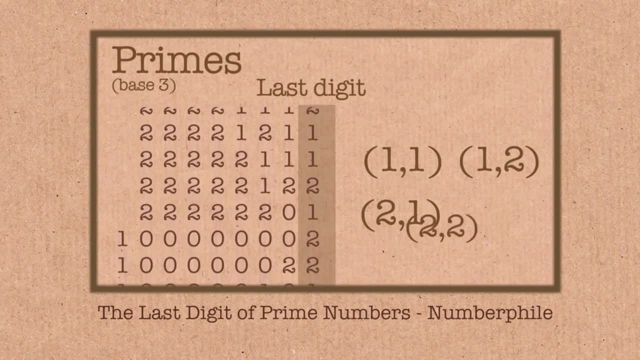 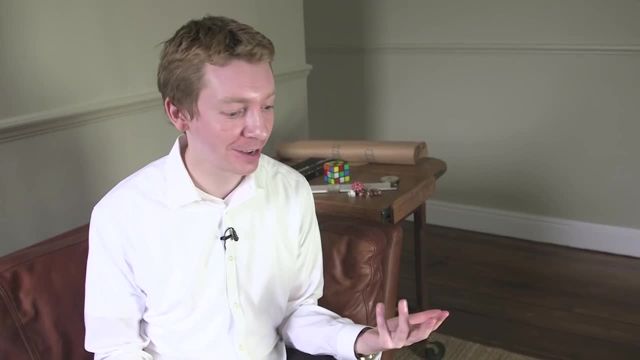 is because, if you remember, there was that prime news, they were looking at primes for consecutive primes. This is what they were looking for. They thought, oh, if primes are random, like coin flips, I'm going to find this effect. 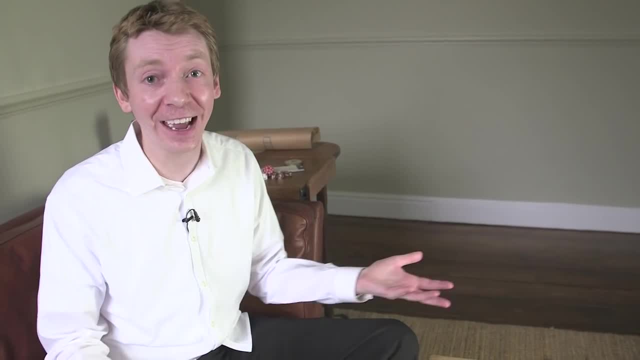 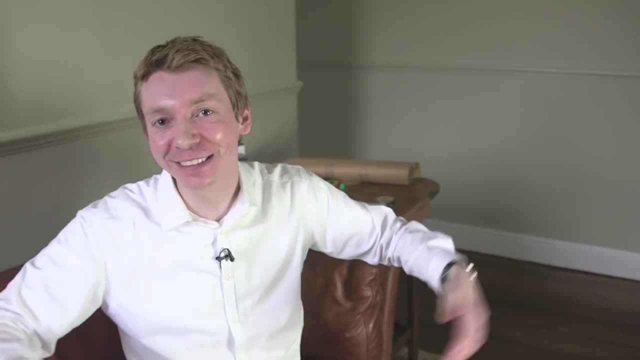 What turned out to be the case is that they didn't find this effect because the primes weren't being random like coins. If you did this forever, if you had a sequence that went on to infinity, the average waiting time then is: I'll show you what that is. 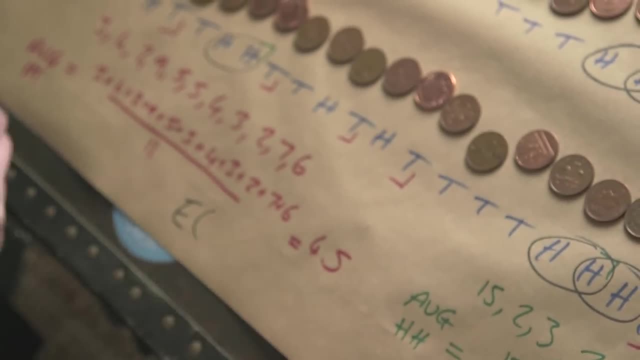 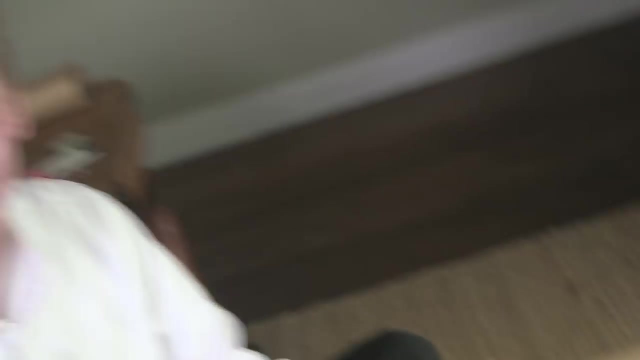 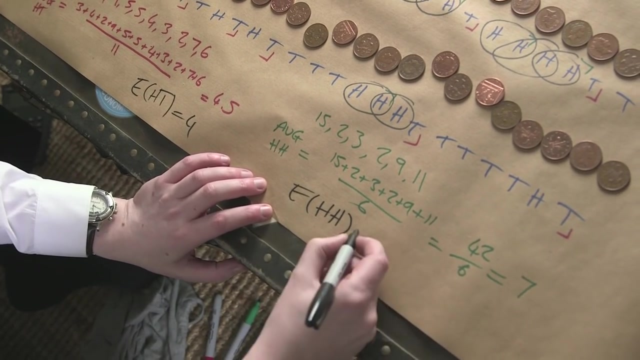 it's called expectation or expected waiting time. The expected waiting time for head tails is equal to four, which kind of makes sense. when it's a quarter probability, That does make sense. And then the expected waiting time for heads- heads- is longer and it's six. 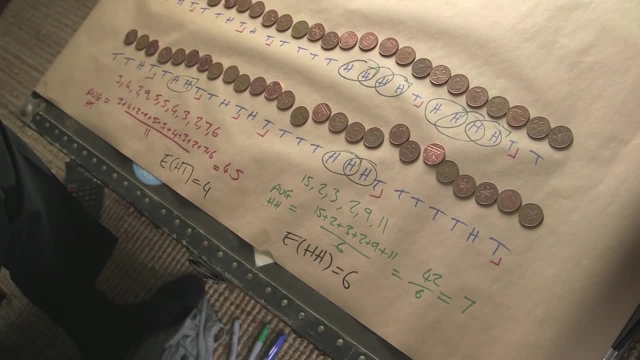 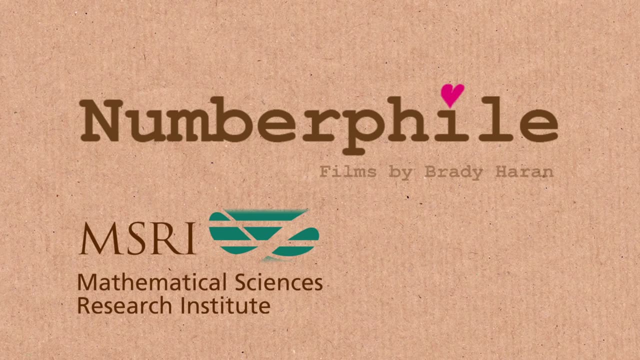 So we were close, but just a little bit off. And if you wanted the expected waiting time for tails, tails, well, that's six as well. That's just the same idea Audible's ever-growing collection has now reached. in the order of: 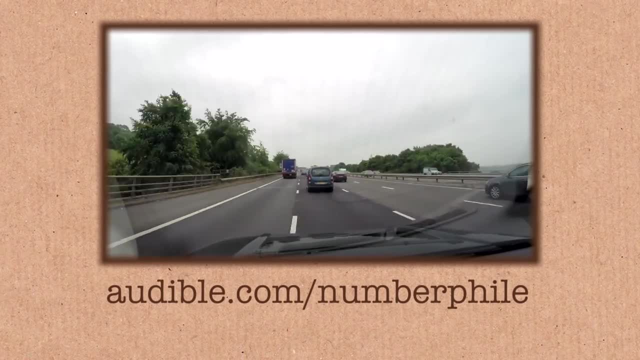 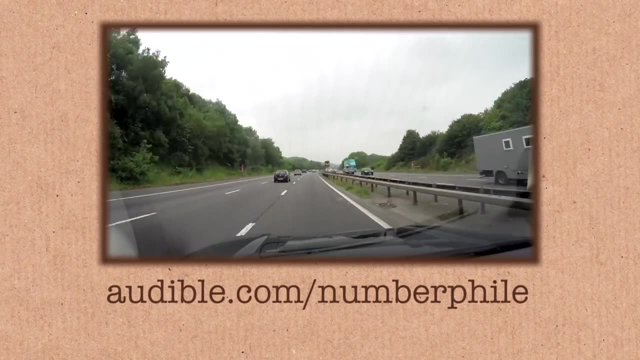 250,000 titles, So no matter what you're interested in, Audible's bound to have multiple options for you. Now I spend a lot of time driving, as you can see here, often in the UK's delightful traffic, And there are few better ways to pass the time. 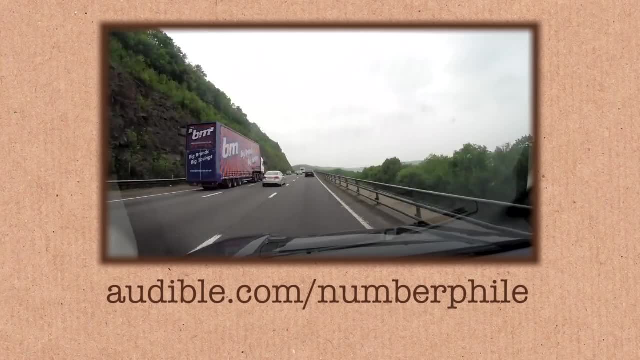 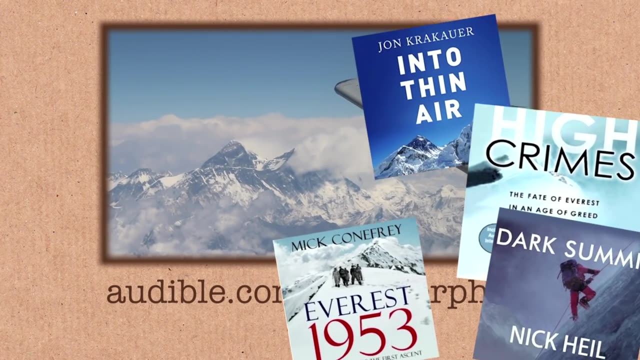 than listening to audiobooks. You can have something entertaining, something educational, or maybe a bit of both. The choice is yours. I particularly enjoy books about mountaineering. I'll put their details in the description, Along with this one about K2,. 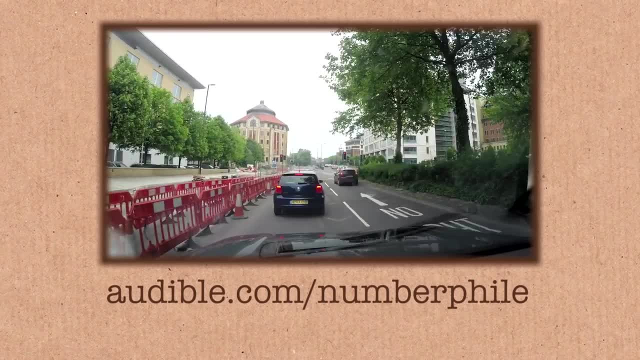 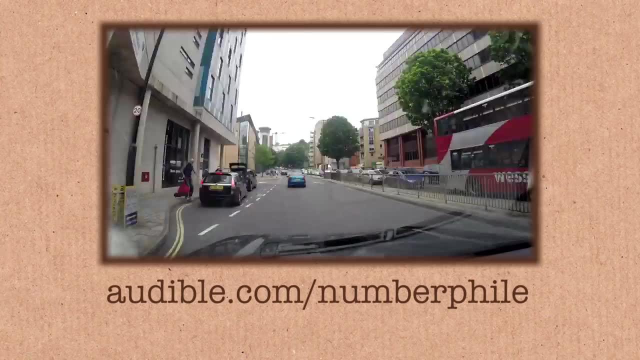 which is one of my favourites as well, And that's just a fraction of the mountaineering books. on Audible, I told you they've got something for everyone. If you'd like to give them a try, go to audiblecom. slash numberphile. 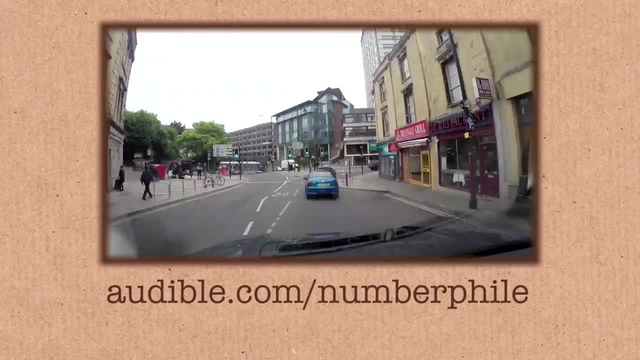 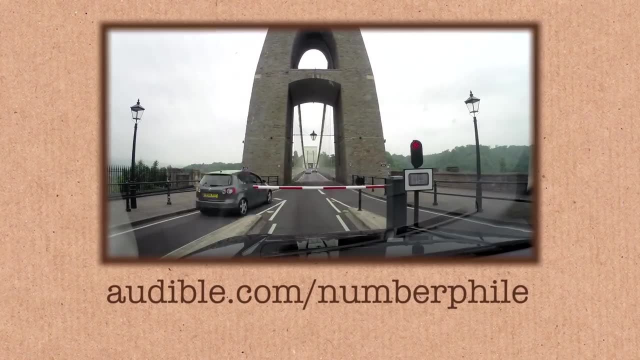 and you can sign on for their free 30-day trial. That trial includes your first book and, as I said, there are plenty to choose from That address again: audiblecom. slash numberphile, so they'll know you came from our channel. 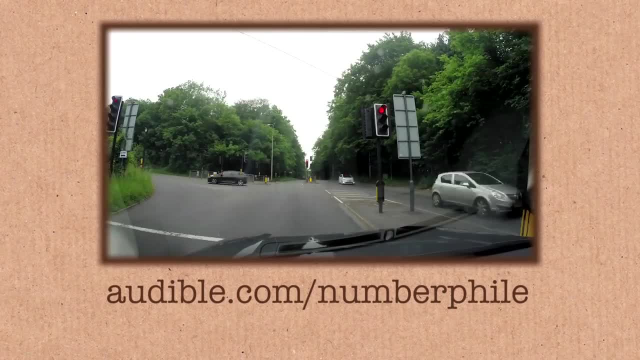 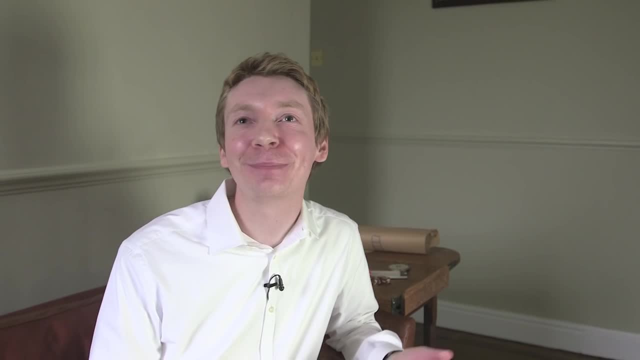 which is handy for us. You can sign up for the trial for 30 days. Our thanks to Audible for supporting this episode of Numberphile. Maths works, Maths just works. It's wonderful that way how maths just works out. 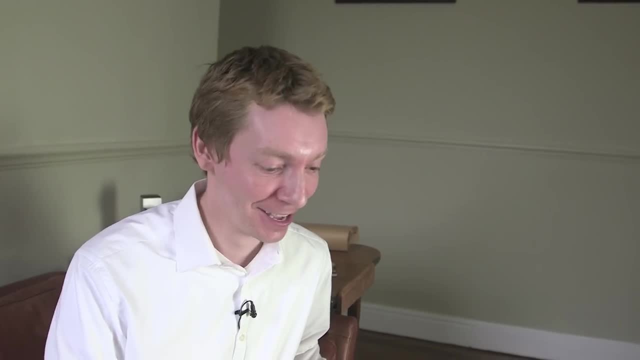 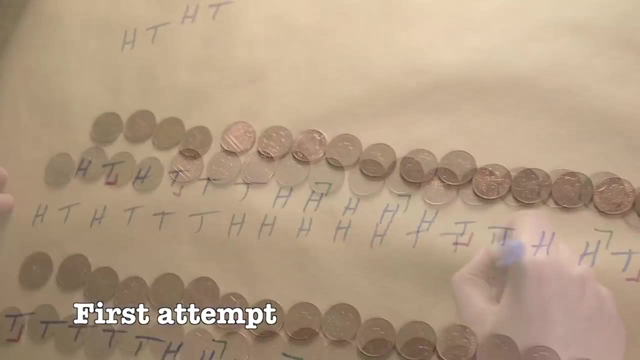 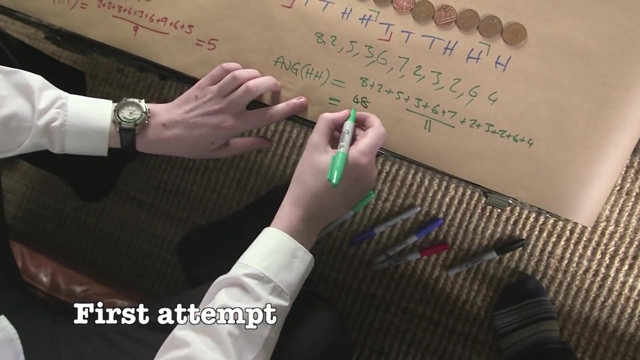 Every time, Every time, just how you want it to work out, Especially with the power of editing What happened. What happened? We did our first take and we got the opposite result from what we wanted. Done yet Over 11,. 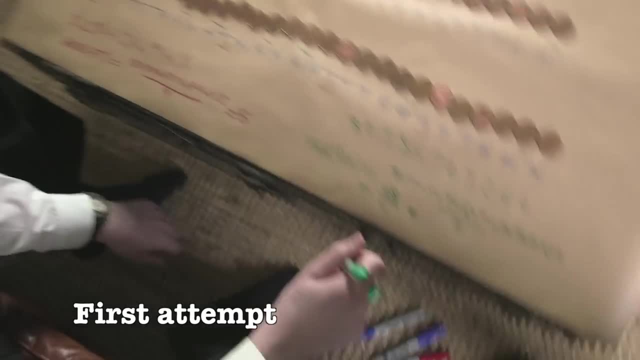 which is the opposite of what I said, And we have to film the whole thing again, right?